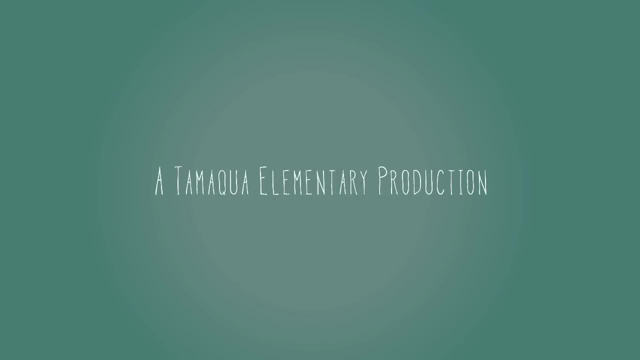 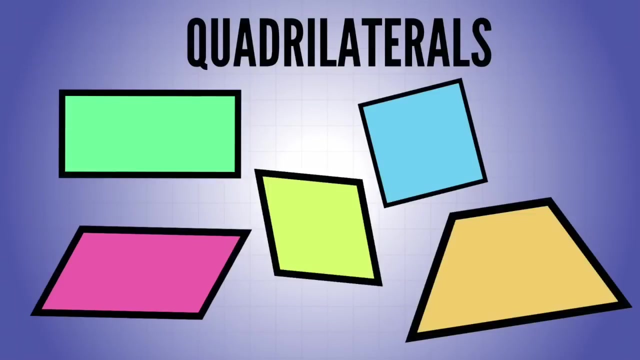 Now we're going to talk about quadrilaterals. Now, quadrilaterals, if we look at the very definition of a quadrilateral, look at the first four letters of quad of quadrilaterals, and that's quad. Quad means four, Laterals means lines. So you're talking about a two. 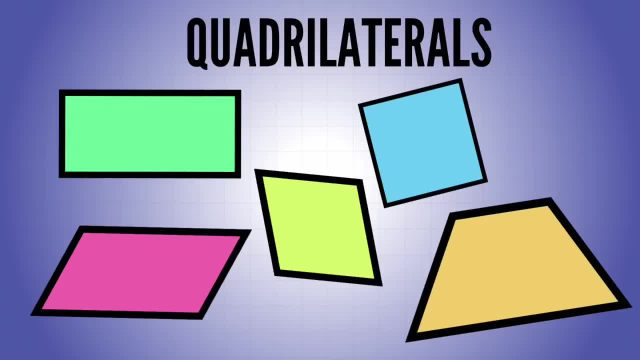 dimensional object shape that has four lines. So what you're seeing here is all different types of quadrilaterals. What is also important is that all the interior angles, when added up in each one of these, add up to 360 degrees- 360 degrees inside of a quadrilateral. That. 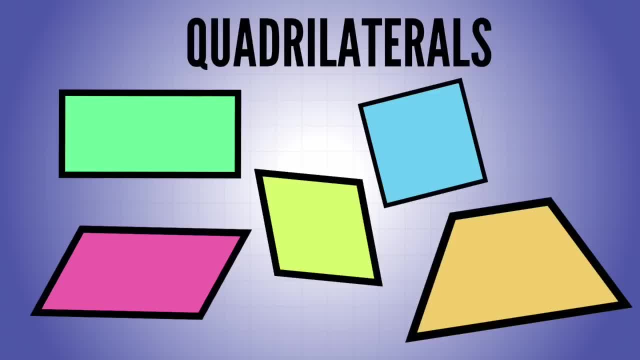 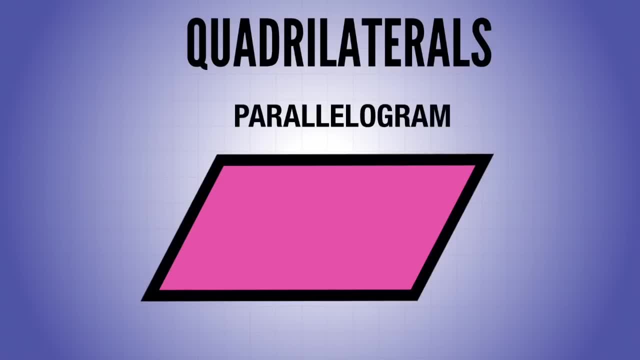 doesn't change, But there are some very important and special quadrilaterals that we're going to be talking about right now. First up is a parallelogram. A parallelogram means that both pairs of opposite sides are parallel. What that means is, if these were extended on forever, they would 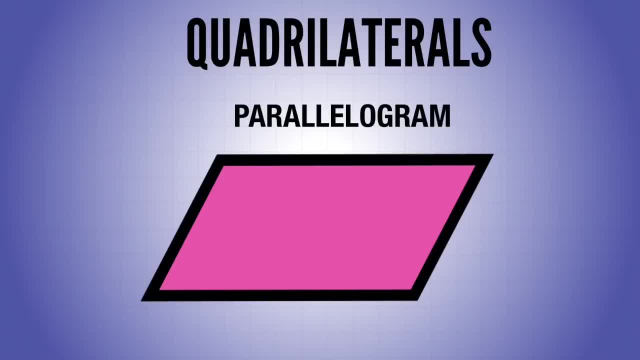 never touch, And the same with these. It also means that both pairs of opposite sides are equal, So these two sides are the same length and these two sides are the same length And, just like I said before, all the angles inside would add up to 360. 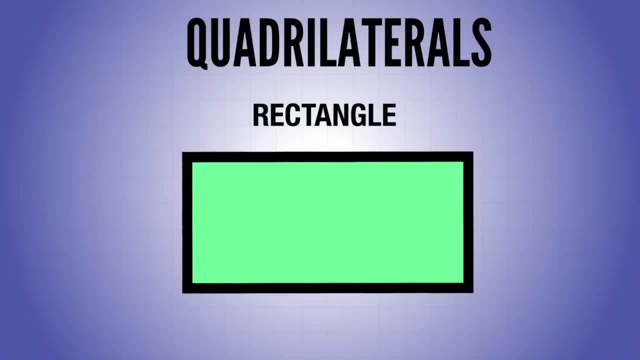 A rectangle is a parallelogram with four right angles. So what that means is this line is parallel with this line and this line is parallel with this line. But it also means that we have our four right angles: One, two, three, four. So that's what makes it a rectangle. 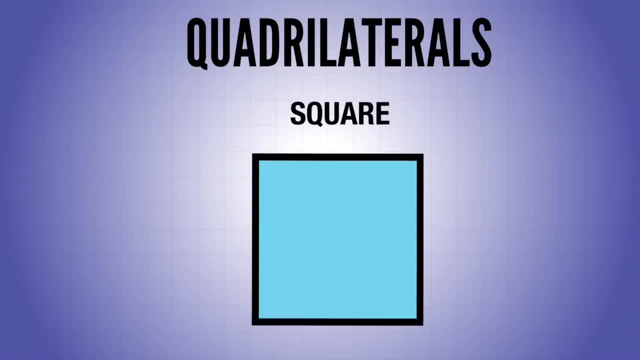 here, A square is a special rectangle. Again, it has the four right angles, It has the two pairs of parallel lines, But it also has all sides. All sides are congruent, are equal. That's where a square really sets itself apart as 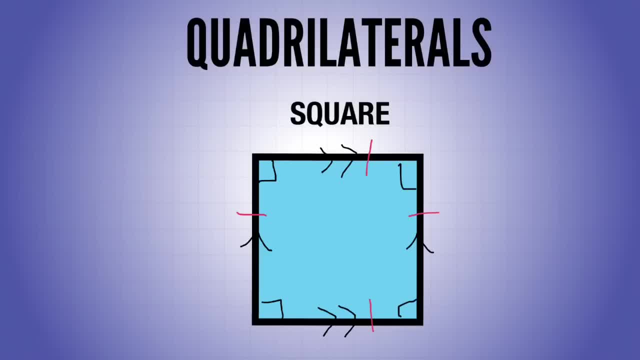 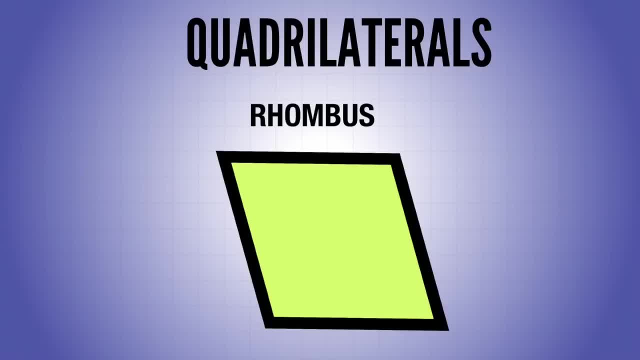 As I mentioned a couple seconds ago, a square can also be called a rhombus. That's because a rhombus is a parallelogram with all the same sides, So that kind of defines a square, other than the square has the 90 degree angles. 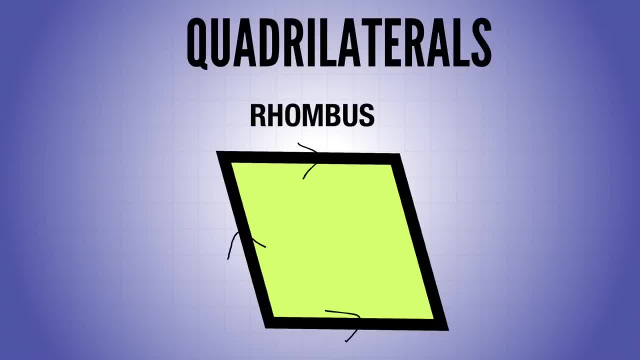 Again, this side is parallel with this side and this side is parallel with this side. All sides are equal. The only difference between the rhombus and the square is that a rhombus doesn't need the 90-degree angles. as you can clearly see. 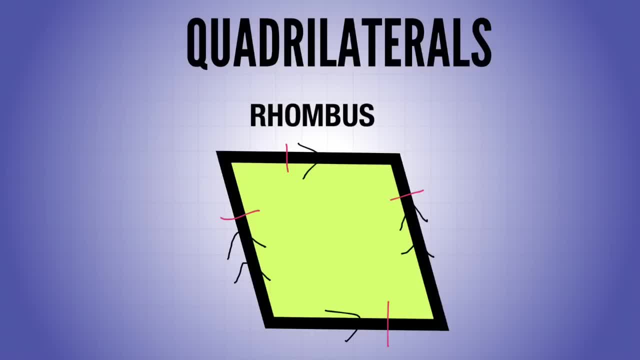 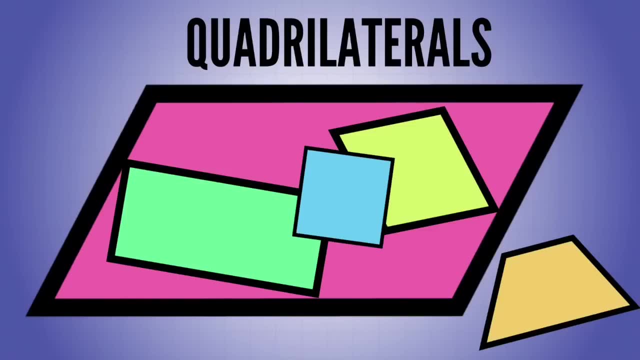 these angles are not right angles, okay, so a square is just a 90 degree rhombus. using this kind of messy diagram that i have here, i'm going to hope to explain you the relationship between the quadrilaterals and the special different quadrilaterals that we looked at today. 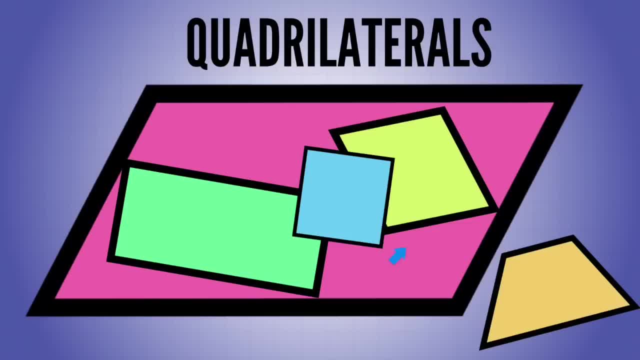 as you can see, the pink is our parallelogram. inside the parallelogram we have three other shapes. that means they're also parallelograms. so this, the rectangle here, the square here and the rhombus are all parallelograms. now remember, parallelograms have two pairs.